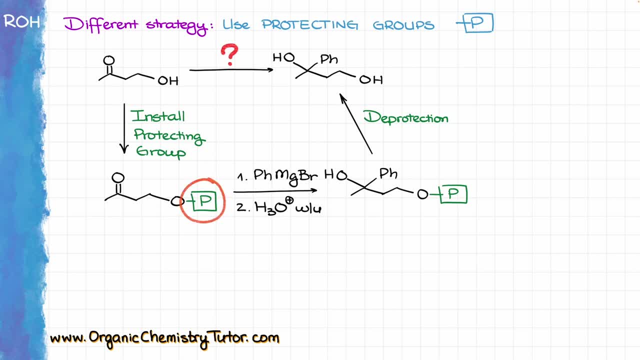 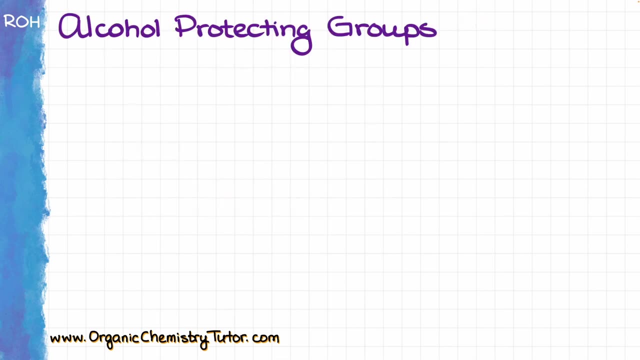 we can use a temporary protecting group that we can put onto our alcohol. This way, alcohol won't be able to mess up our reaction And once we're done we can take that protecting reagent off and get our original functional group via the deprotection step. There are 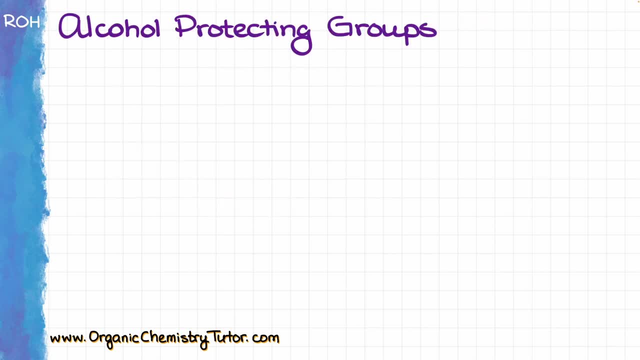 three common types of protecting groups that we use for alcohols. That's going to be the silyl protection, the benzyl protection and the acetyl protecting groups. Each of these protecting groups has its strengths and weaknesses, and the most universal of all. 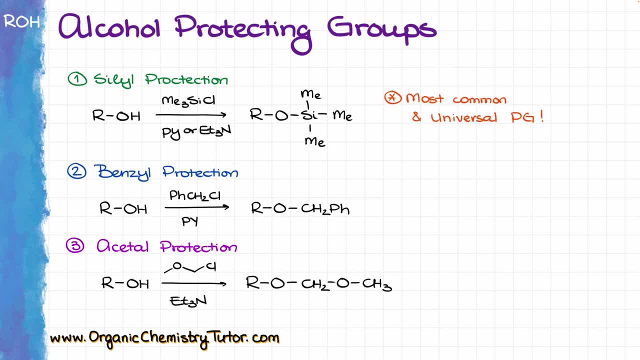 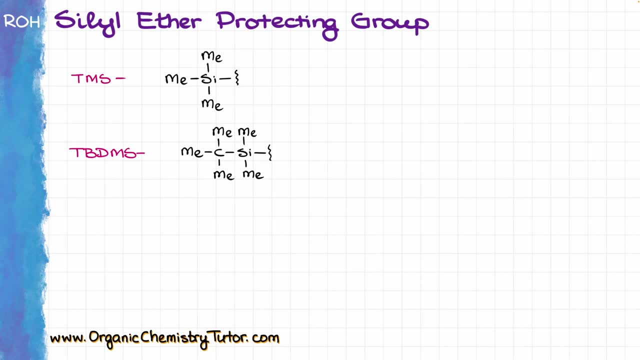 of those three is going to be the silyl protection group, so let's talk about that one first. When it comes to silyl ether protecting groups, the most two common silyl ethers that you are going to be using is either going to be trimethyl silyl ether- 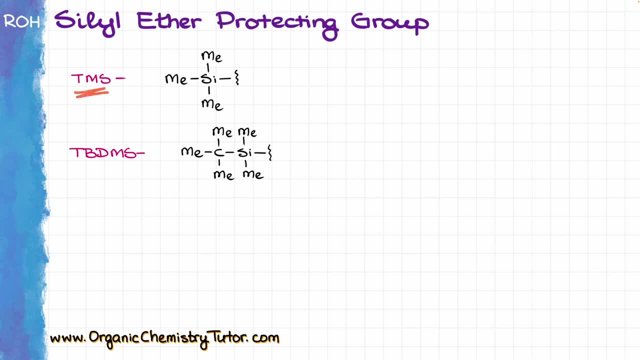 or TMS for short, or we're going to be using 3-butyldimethylsilyl ether, which we're going to abbreviate as TBDMS. We use the second one, this guy, when we want to turn our alcohol into a more bulky group, for finer steric control of our reaction. This one also. 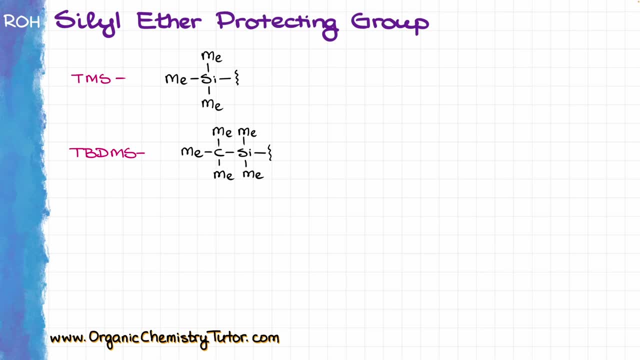 seems to be a little bit more resilient to various reaction conditions. For our purposes, however, these are interchangeable, so I'm going to be using the TMS as an example structure here for all of my reactions, And the first question that I have is: how are we going to apply our protecting 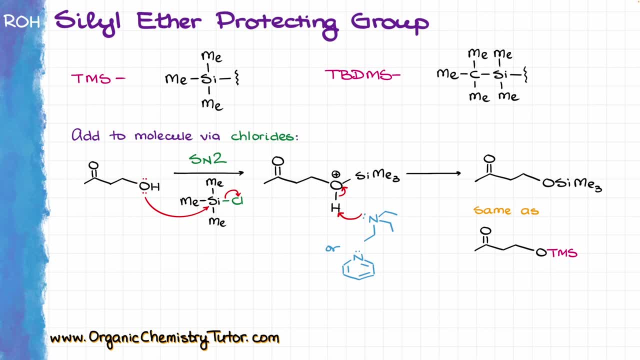 group onto our molecule. In the case of the silanes, we are going to use the corresponding chloride. so if I wanted to add TMS to my molecule, I would use the corresponding trimethylsilane chloride in pyridine or triethylamine as a solvent. The mechanism here is fairly straightforward. 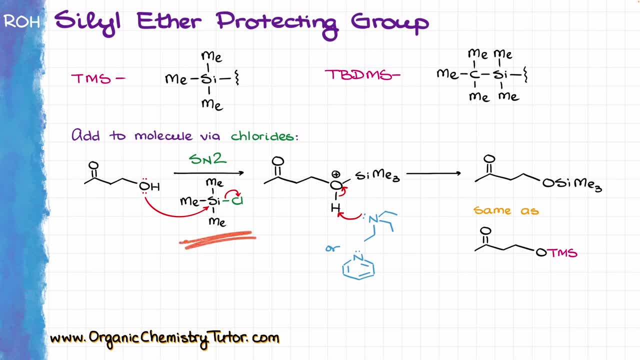 This is going to be an SN2-style reaction, where first alcohol is going to displace the chlorine out of my silane, giving me a protonated intermediate, and then we are going to be using one of our bases, either triethylamine or maybe pyridine, which we typically can use as our solvent. 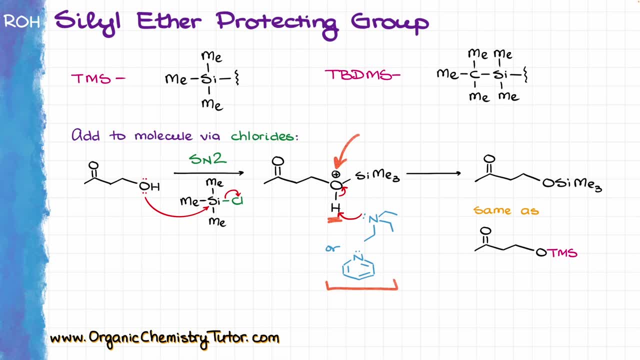 to deprotonate that molecule and give us a neutral product. We can spell out our trimethylsilane group as such, or, if we are pressed for time, or maybe you just like abbreviations, you can abbreviate that as TMS. The big limitation of this protecting group is: 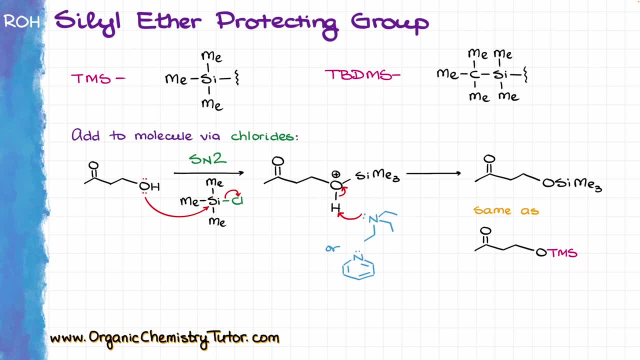 in the case when you have multiple potential nucleophilic sites. In this case, you can potentially find yourself in a situation where you have silicon sitting on multiple places in your molecule. So when you are planning your synthesis, it is always a good idea to introduce. 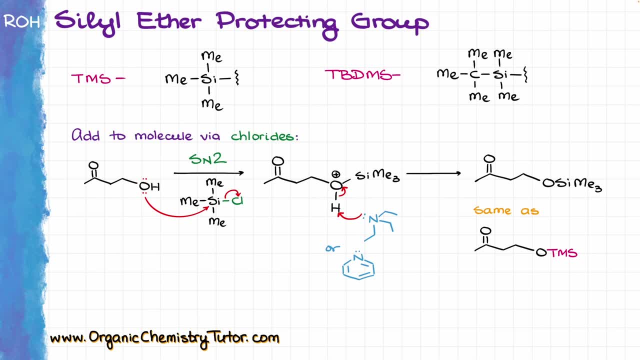 your protecting group at an appropriate point where it is not going to jump on multiple atoms just making a mess. It's hardly going to be an issue with simple molecules, of course, but it can certainly muddle the waters in more complex substrates. 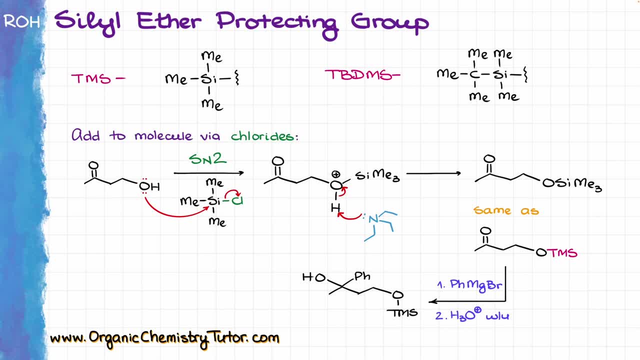 And so now, when I have my alcohol protected, I can easily do my reaction and not worry about alcohol messing things up. Alright, cool. so we've done our chemistry here. everything worked the way we anticipated. now what We still have- this protecting group, this TMS, sitting on our molecule. 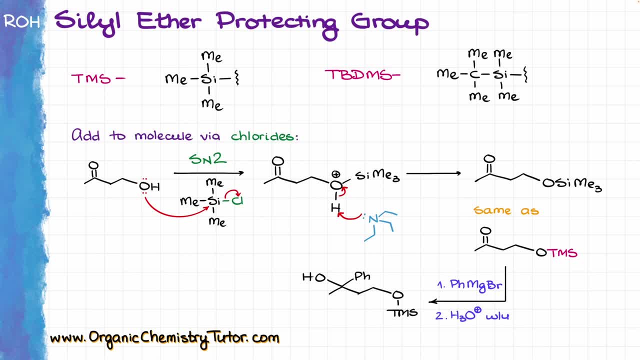 so we need to get rid of it somehow And, as I've mentioned before, silyl protection is incredibly resilient to a lot of different conditions. This means that it's going to stay put in both acidic and basic conditions, So does it mean that we are stuck with it forever? Well, certainly not. 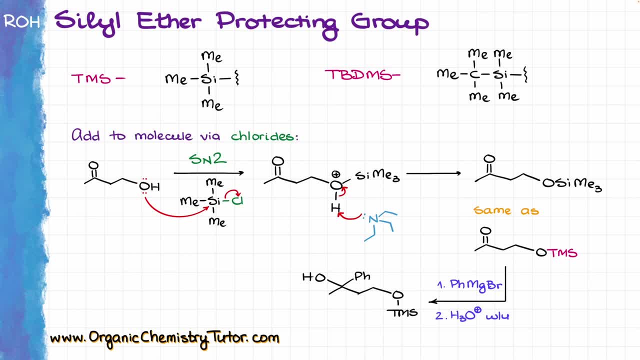 While the silyl protecting group might be very resilient, it does have one major weakness, and this weakness is the fluoride ion. If we treat our product with anything containing fluoride, it will react with silicon and displace it via a simple SN2-style reaction, The easiest source. 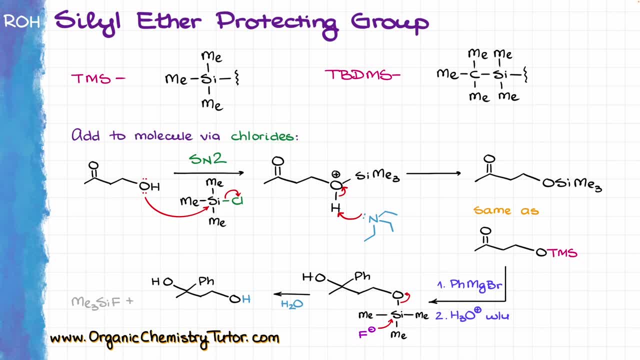 of a fluoride is, of course, going to be hydrofluoric acid, HF. However, since the glass square that we use in the lab is a little bit smaller, it's not going to be as good as the fluoride ion, so we are going to have to do something about it. So, unless you have platinum beakers in your lab, 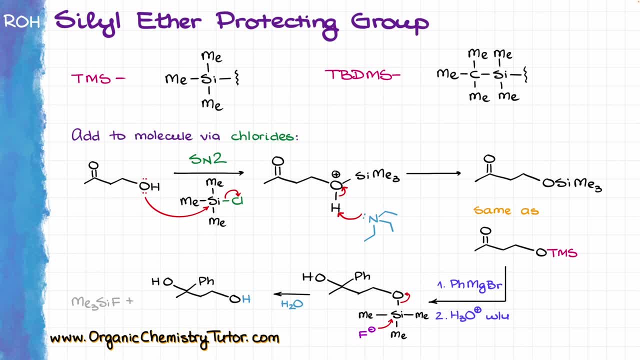 and yes, they do exist. you are out of luck and need some other source of fluoride. Ionic fluorides like, let's say, something like potassium fluoride or something similar, have one major problem: They do not dissolve in organic solvent. So we need to do something more creative to kill both birds on the same stone. 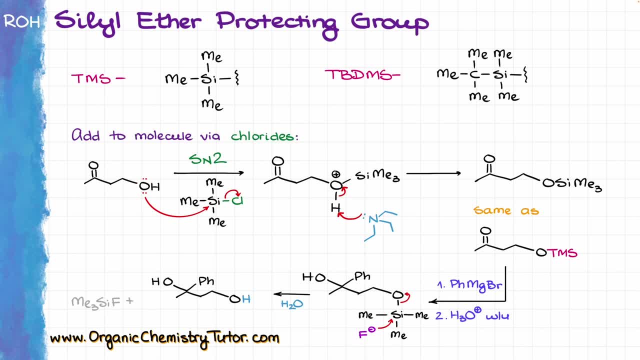 Bring fluoride to our molecule and have it in an organic solvable form, And the solution here is quite elegant: To make our ionic fluoride solvable in organic solvents, we are going to use organic cations as our counter ions. The two most common ones are going to be tetraethylammonium fluoride. 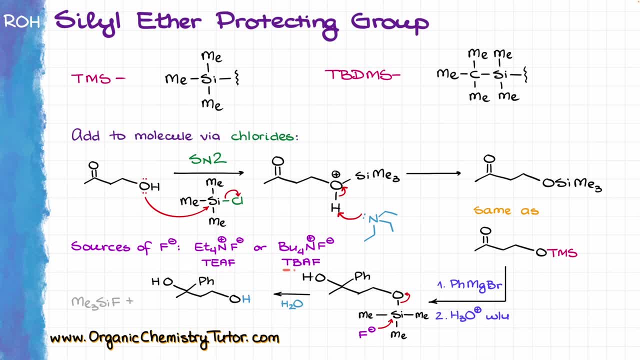 or TIF, and another one is going to be tetrabutylammonium fluoride, or TBF. These reagents are quite soluble in organic solvents and they will drag the fluoride ion with them into our solution, delivering it to where it needs to be and where it needs to act upon our molecule. 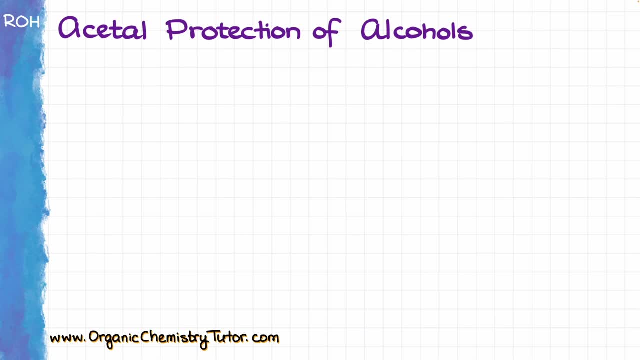 Now, as I've mentioned at the beginning of this video, silyl protection is one of the three main protecting groups that we typically see for alcohols. The next method that we are going to see sometimes is the use of acetyls. Typically, we're going to see either a dihydropyrane, DHP, 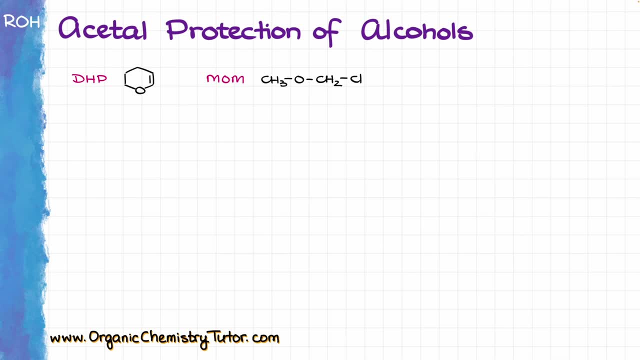 or methoxymethyl or dihydroxychloride or dihydroxychloride or dihydroxychloride. We add DHP group onto the alcohol in acidic conditions. This is a typical electrophilic addition to an alkene reaction. In this case the alkene is especially susceptible. 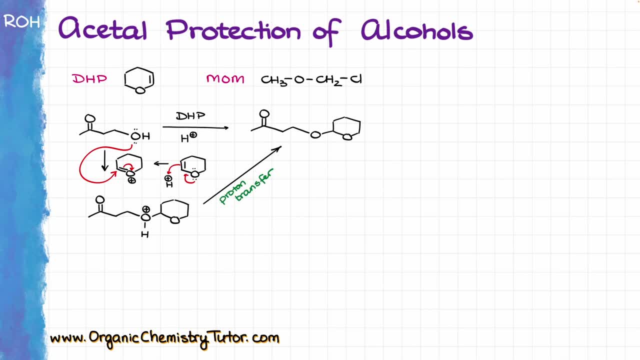 to this reaction due to the polarization from the oxygen atom. Once the protecting group is on, it is very resilient towards the basic conditions. However, it is sensitive to acids like any other acetyl, and it will easily pop off in acidic conditions. 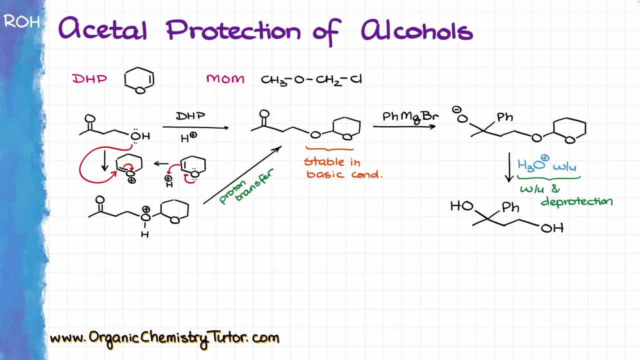 This is especially convenient since we can often combine the deprotection step and the workup after reactions like, let's say, a Grignard reaction. So in this case I can accomplish both in a single synthetic procedure by protonating everything that needs to be protonated. 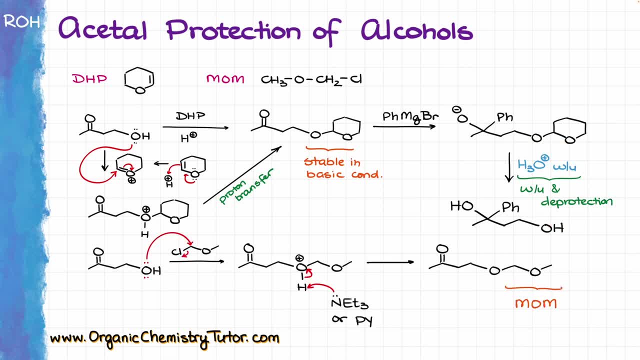 and taking my protecting group off. So when it comes to methoxymethyl protecting group, that one is installed in a similar fashion to the silyl protecting groups- Basic conditions via the SN2- and similar to the DHP, the MOM is going to be sensitive towards acid and will easily pop off. 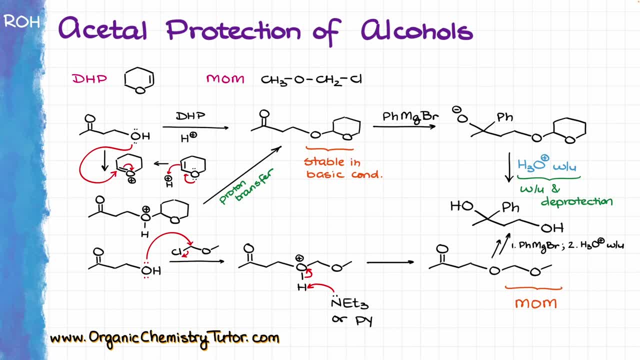 in acidic conditions. I also want to point out that if you opt to use one of these two protecting groups, you should probably go with DHP, unless your substrate is really sensitive towards acids. The thing is, while MOM is an excellent protecting group, the reagent that we are using here, 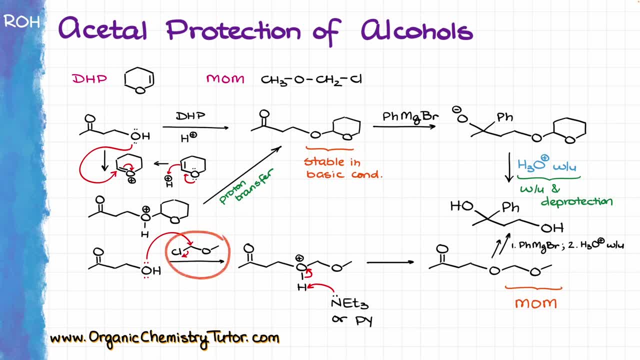 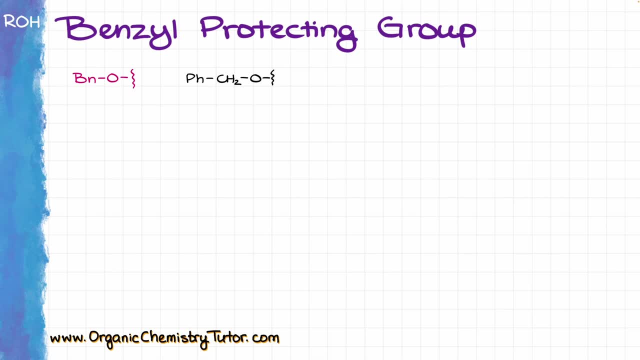 MOM chloride. well, that one is quite toxic and carcinogenic, So you should definitely avoid this MOM at all costs. And finally, we have the benzyl protecting group. This is an incredibly resilient protecting group and we often see that when we are dealing with the glycochemistry. 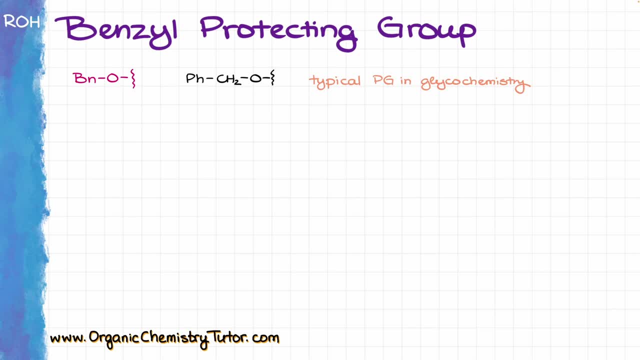 which is chemistry of carbohydrates. So most likely you are going to be using that as one of your major protecting groups if you cover sugars at the end of your second semester. Typically we are going to install the benzyl protecting group via an SN2 reaction of the 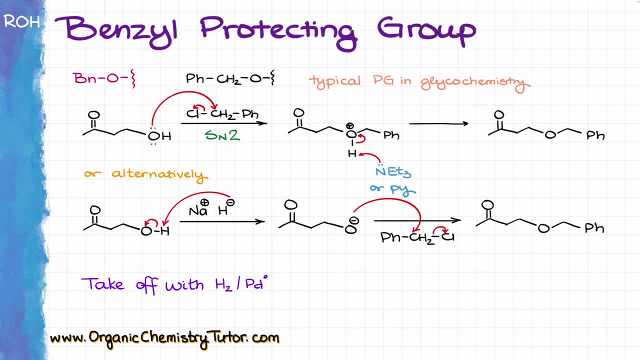 corresponding alkoxide and benzyl halide. This is a typical Williamson ether synthesis, so there is nothing special about this reaction. However, you can also do it in milder conditions when the SN2 reaction happens within alcohol itself, due to an extremely high reactivity of 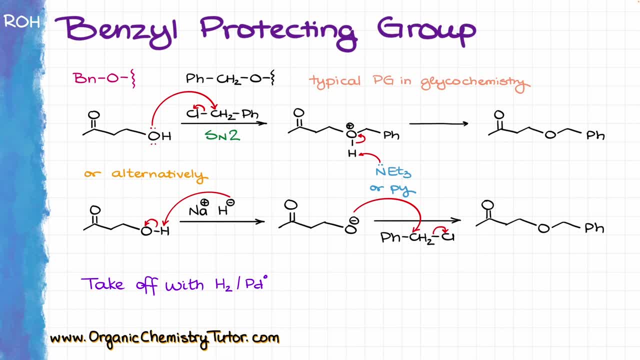 the benzyl chlorides, And, just like in the case with MOM, benzyl chlorides and bromides are incredibly toxic and carcinogenic, so you should avoid those at all costs, if you can, of course. What's really cool about this protecting group is that it's bulky and chemically resilient. 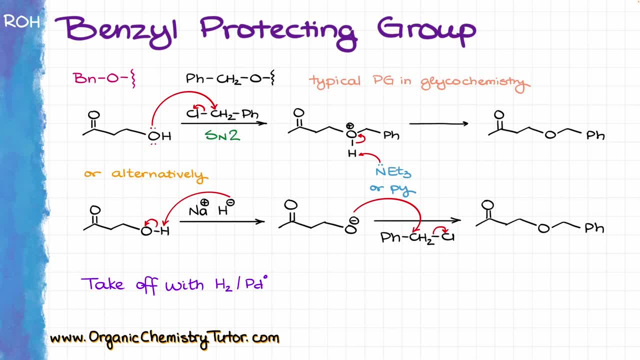 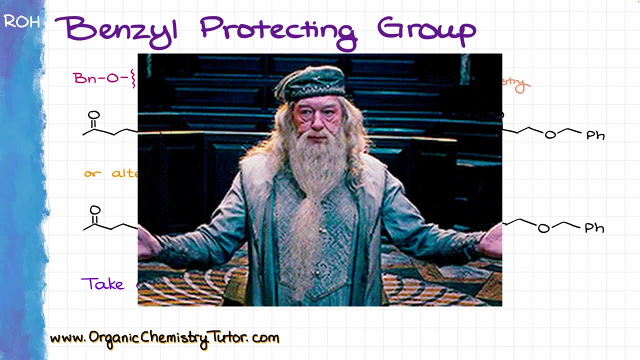 so you are going to be more or less safe using it in both basic and acidic conditions. However, we can easily take it off by using hydrogen on palladium catalyst. Generally, we use this type of chemistry when we want to reduce a double or a triple bond. however, benzylic position, just like 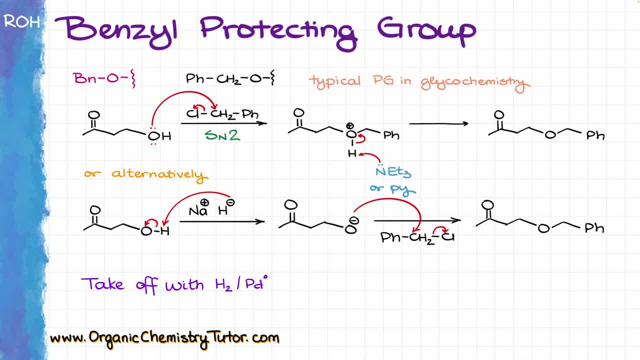 Albus Dumbledore has its own privileges And if you have a CO bond in the benzylic position it can be broken by a single bond. So if you have a CO bond in the benzylic position it can be broken. by a single bond. However, if you have a CO bond in the benzylic position, it can be broken by a single bond. However, if you have a CO bond in the benzylic position, it can be broken by a single bond.